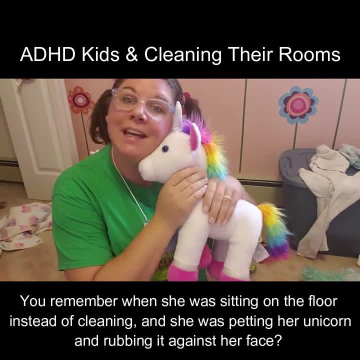 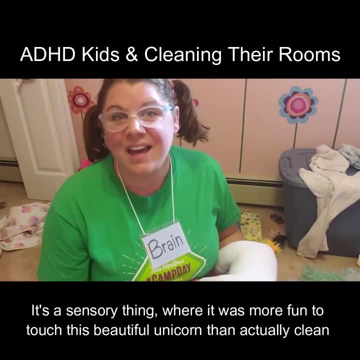 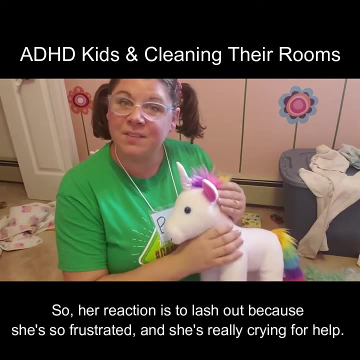 instead of cleaning, and she was petting her unicorn and rubbing it against her face. It's a sensory thing where it was more fun to touch this beautiful unicorn than actually clean, because her brain- me- didn't know where to start, So she fixated on something she does like. 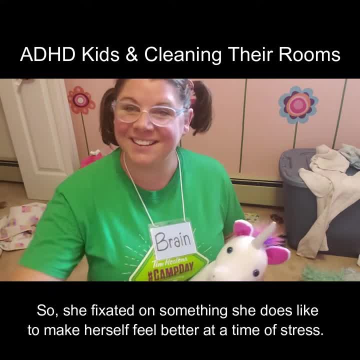 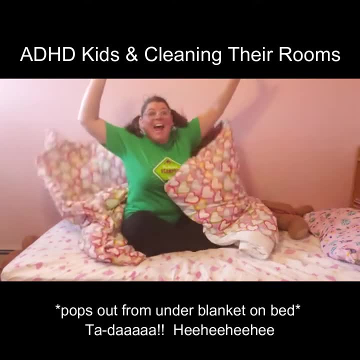 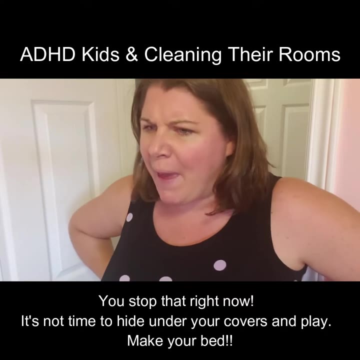 to make herself feel better in a time of stress. I'm going to come back in two minutes. Where's Laura? Stop that. right now It's not time to hide under your covers and play Make your bed. Do you remember when Laura popped out from underneath the covers and laughed hysterically? 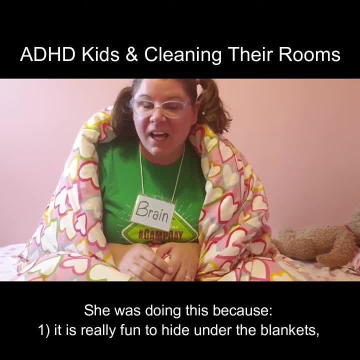 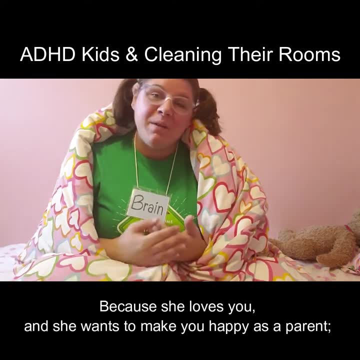 She was doing this because: one, it is really fun to hide under the blankets and way more fun to do this than to clean. Two, she was trying to make you smile and laugh because she loves you and she wants to make you happy as a parent And, unfortunately, cleaning is not something that her brain 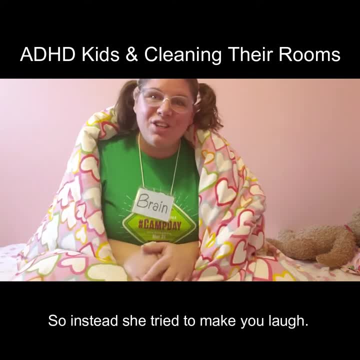 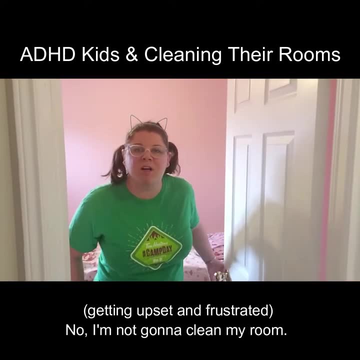 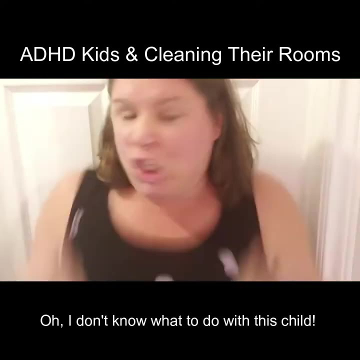 will let her do yet. So instead she tried to make you laugh. I'm very disappointed in you. Yeah, yeah, No, I'm not gonna clean my room. Oh, I don't know what to do with this child. Remember how she shut this door and screamed at you some profanities. 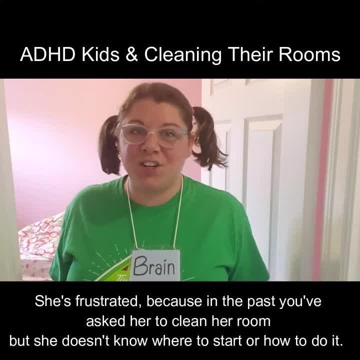 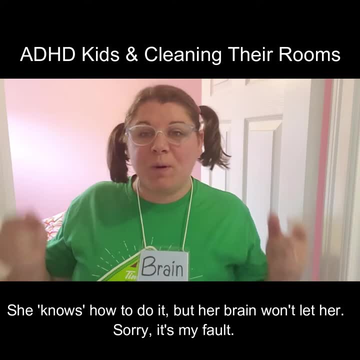 She's frustrated because in the past you've asked her to clean her room, but she doesn't know where to start Or how to do it. She knows how to do it, but her brain won't let her. Sorry, It's my fault. 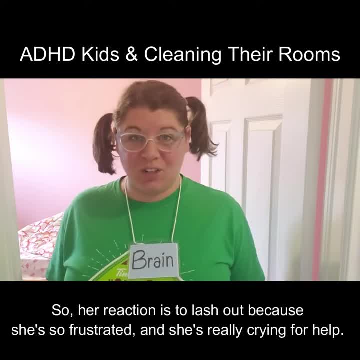 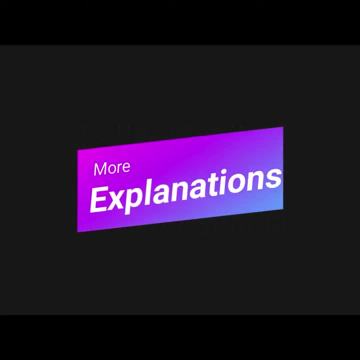 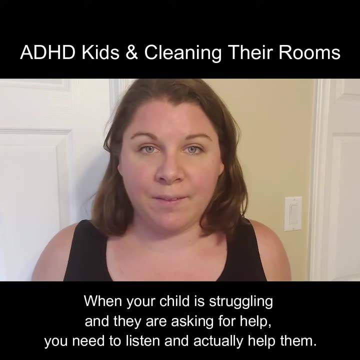 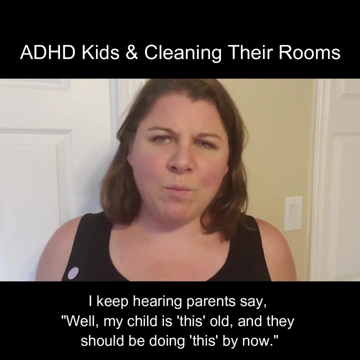 So her reaction is to lash out because she's so frustrated and she's really crying for help. Parents, I cannot stress this enough: Your child's struggling and they're asking for help and you need to listen and actually help them. I keep hearing parents say: well, my child is this old and they should be doing this by now. 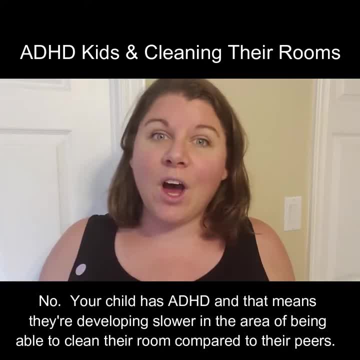 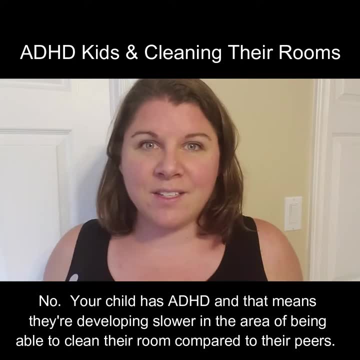 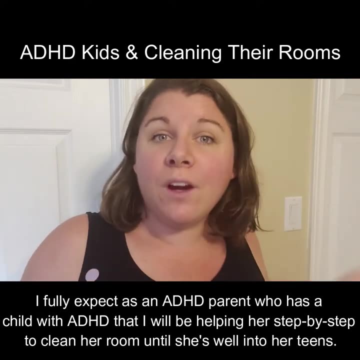 No, your child is ADHD and that means that they are developing slower in the area of being able to clean their room compared to their peers. I fully expect, as a ADHD parent who has a child who has ADHD, that I will be helping her step by step to clean her room. 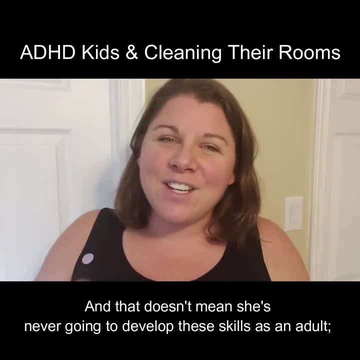 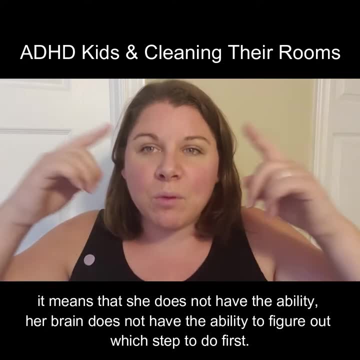 until she's well into her teens. and that doesn't mean that she's never going to clean her room, going to develop these skills as an adult. it means that she does not have the ability, her brain does not have the ability to figure out which step to do. 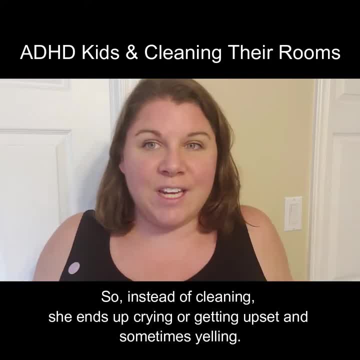 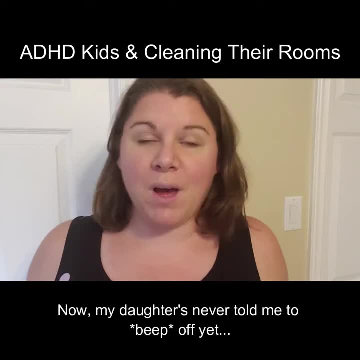 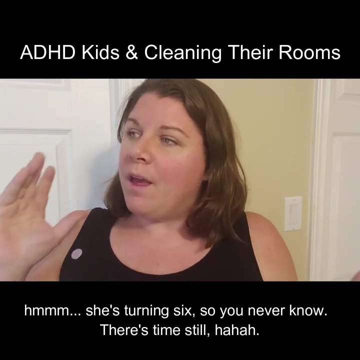 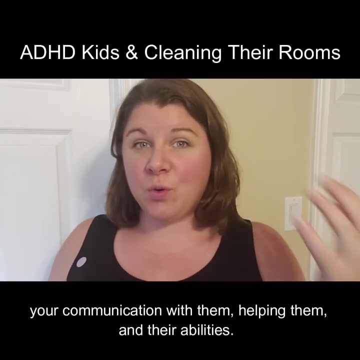 first. so instead of cleaning, she ends up crying or getting upset and sometimes yelling. now my daughter's never told me to beep off, yet she's turning six, so you never know where there's time still, but if your child's at the point of screaming at you, that means there's been a disconnect between your communication. 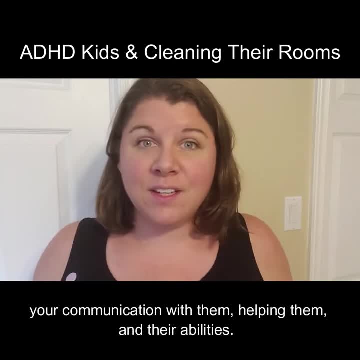 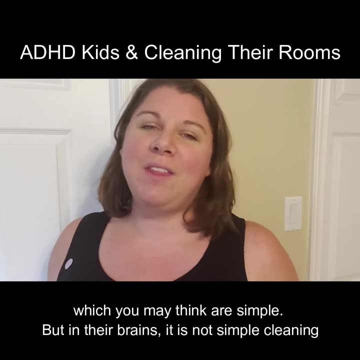 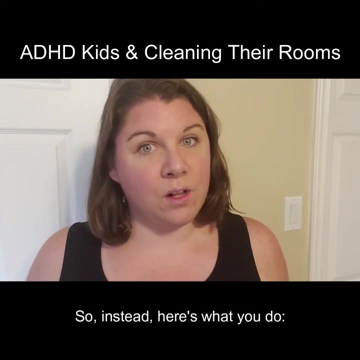 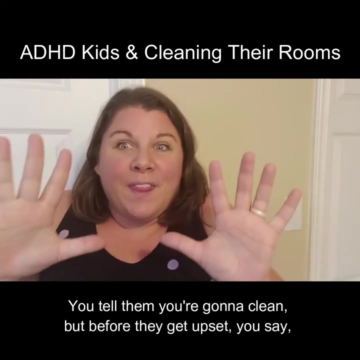 with them, helping them and their abilities. stop, stop expecting them to be able to do these huge tasks, which you may think are simple, but in their brain it is not simple. cleaning, trust me, I still struggle you. so instead, here's what you do: you tell them you're gonna clean, but before they 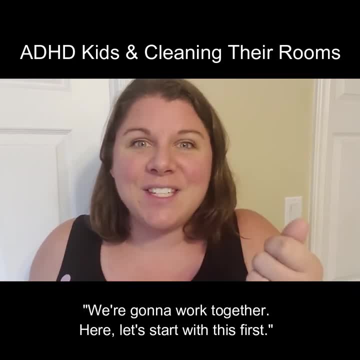 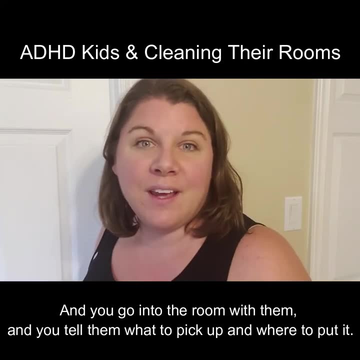 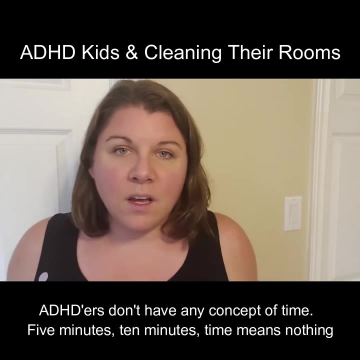 get upset, you say: we're gonna work together here, let's start with this first. and you go into the room with them and tell them what to pick up and where to put it and, before they get overwhelmed, direct them to the next piece. don't tell them I'll be back in five minutes. ADHDers don't have any. 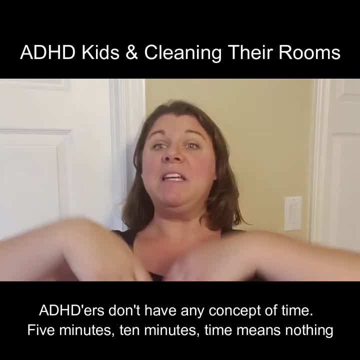 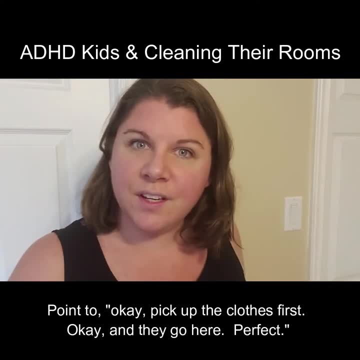 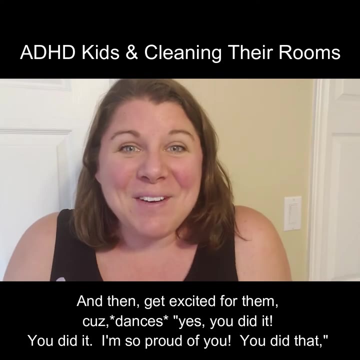 concept of time. five minutes, ten minutes time means nothing, so stay with them, help them. point two: okay, pick up the clothes first, okay, and they go here, perfect, and then get excited for them cuz, yes, you did it, you did it. I'm so proud of you. you did that and watch them change, watch them get. 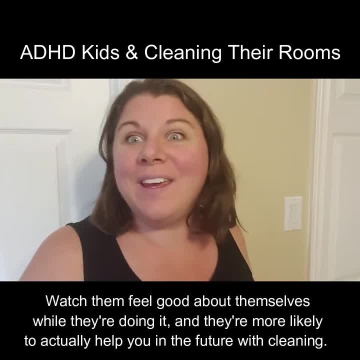 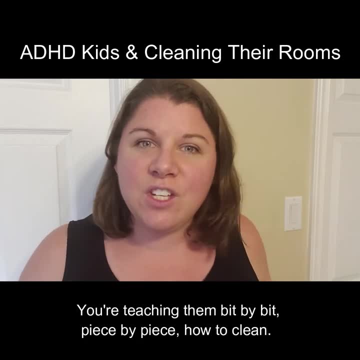 excited. watch them feel good about themselves while they're doing it and they're more likely to actually help you in the future with cleaning. you're teaching them to feel good about themselves. you're teaching them, bit by bit, to learn to clean themselves. you're teaching them, bit by bit, to learn to clean. 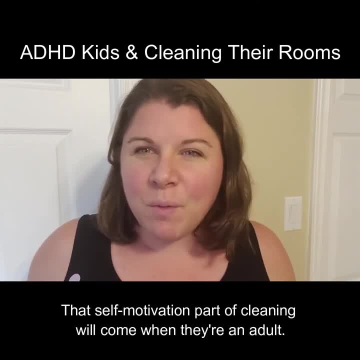 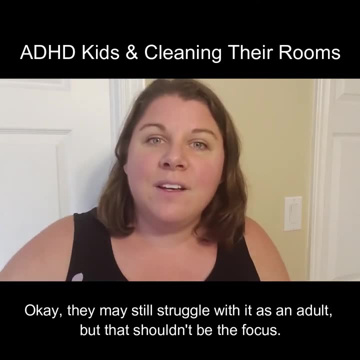 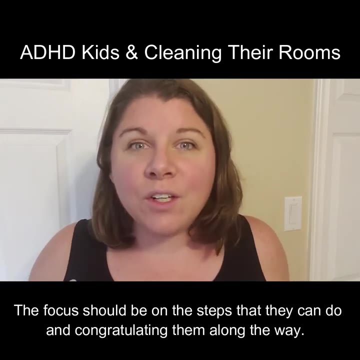 bit, piece by piece, how to clean that self-motivation. part of cleaning will come when they're an adult. okay, they may still struggle with it as an adult, but that shouldn't be the focus. the focus should be on the steps that they can do and congratulating them along the way. parents, I really hope this helps, please.